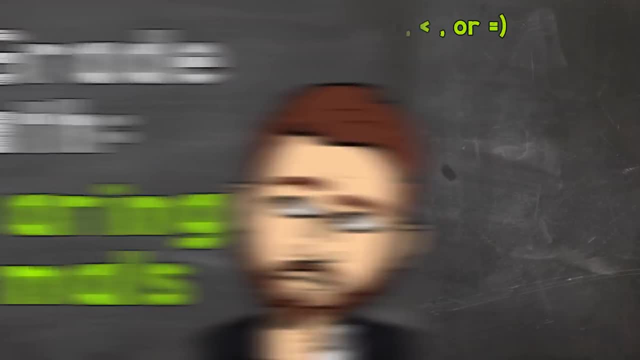 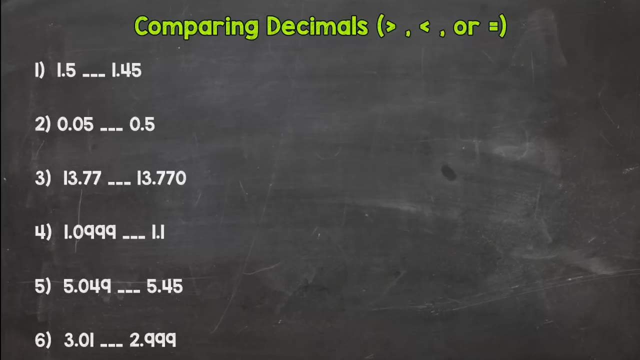 Welcome to the comparing decimals video. So this is going to be an instructional video on how to compare decimals and then we will follow this up with a mastery check where you try some on your own to see if you have it down. I highly suggest you check out the equivalent decimals instructional video on mastery. 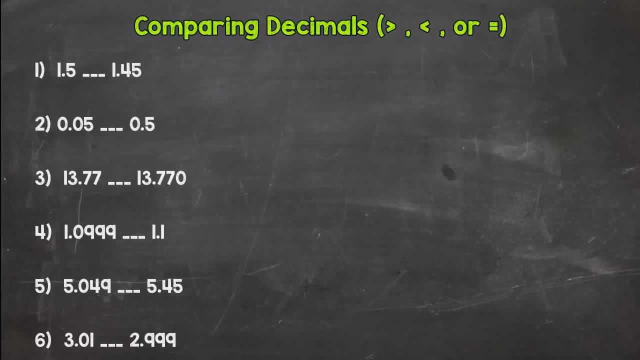 check. before moving on to comparing decimals, I drop the links to those in the description. If you're already familiar with equivalent decimals, then you should be good to go, but when I say the words equivalent decimals and you have no idea what that means, definitely check those. 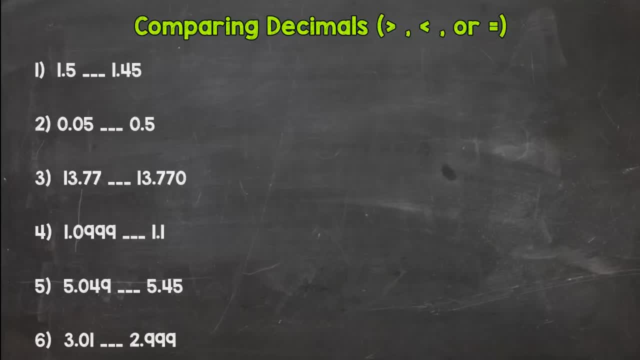 videos out first and then come back to comparing decimals. So I put six numbers here and basically we're just going to go through some examples and then you're going to try some on your own. So number one: here we have one in five tenths and 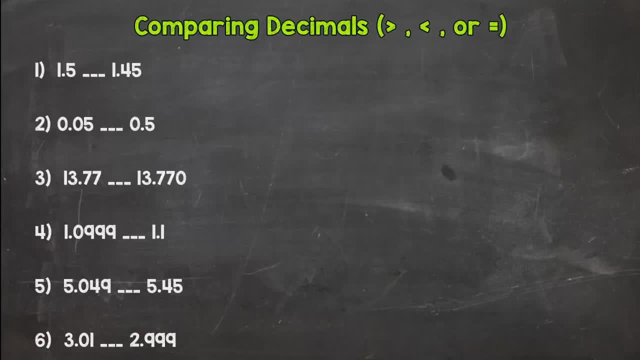 one in forty five hundredths When we compare decimals. when we're first starting out, we're gonna line up our decimals to make sure we're comparing these properly. Line up our decimals and that will line up all of our places for us. Now, after we line up, 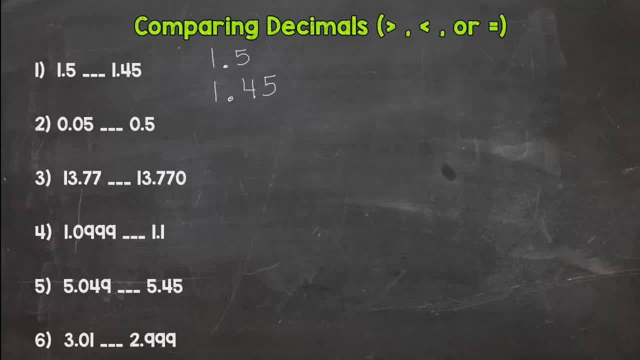 our decimals. you should notice we're kind of offset a little bit. This one only, the top one only goes to the tenths and the bottom one goes to the hundredths. So after watching the equivalent decimals video or knowing what equivalent decimals are, you know you can add a zero or put a zero. 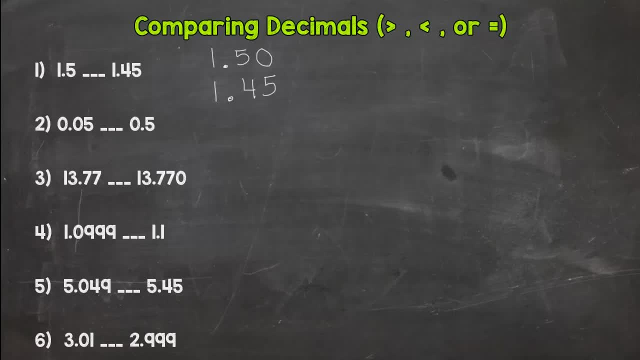 placeholder zero to the right of the five, so both of our numbers go to the hundredths place. That's going to make it easier to compare and order when we get to ordering decimals. So now we both so line up our decimals, put placeholder zeros in if necessary. Now we need to look left to right and compare to the. 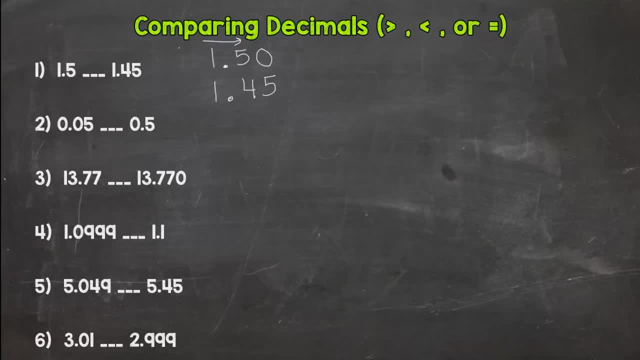 greatest value place and work our way to the right to least value place if we have things in common. So, for example, let's look at our ones place. we have a one and we have a one, so we can't compare. they're the same there. So let's. 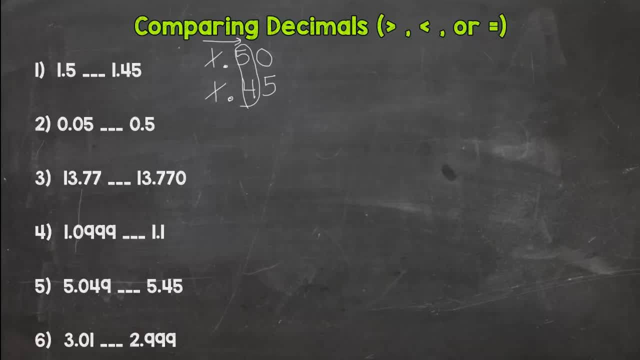 look at our tenths place. Can we compare this place? Yes, the five is greater than the four. Okay, so this is automatically greater. one and five tenths is greater than one in forty five hundredths. Now, here's a common mistake here. I'm going to rewrite them over here. Do not say: one in forty five hundredths is. 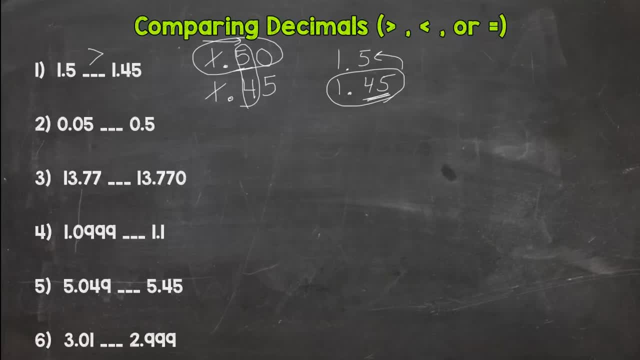 greater than one in five tenths because it has more numbers. That doesn't matter. when we get to decimals You need to go left to right and go place by place. This tenths place holds more weight than anything to the right of it, So you go. 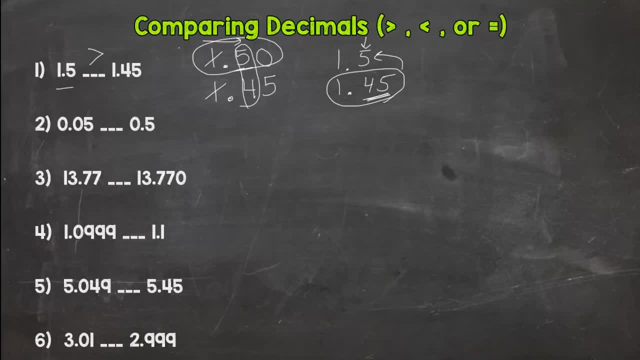 left to right, And then you should be able to say this comparison sentence from left to right and you would read it: one in five tenths is greater than one in forty five hundredths. So let's line up number two here. Let's line our decimals up. We have 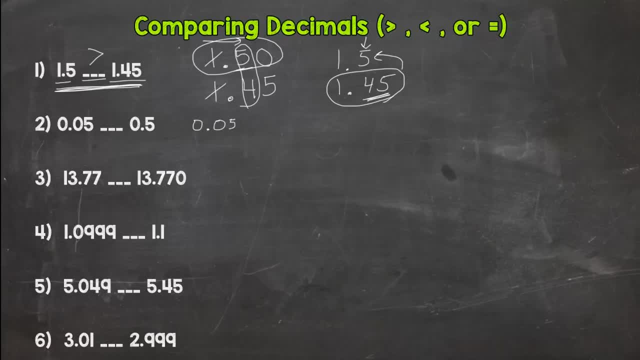 one or, I'm sorry, we have five hundredths compared to five tenths. Look left to right. You might know which one's greater right away, but you need to to be able to explain why and in what place do you look in order to compare. 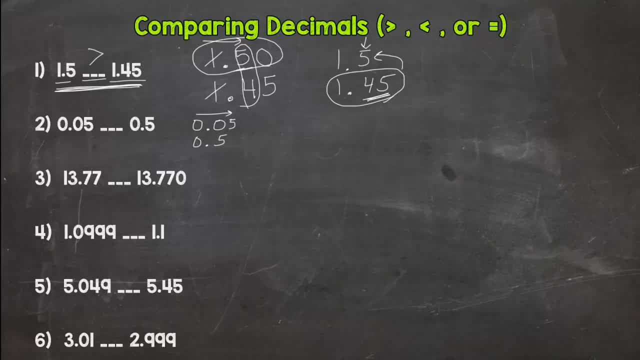 these and then read the comparison sentence from left to right. So let's check here. Let's look left to right. We don't have any holes, so we can't compare that. Let's look at our next greatest valued place, which is the tenths, Can we? 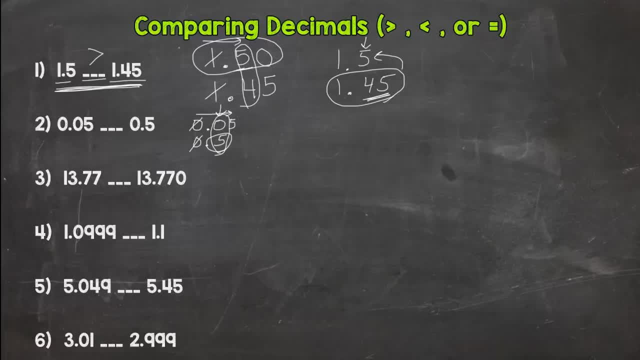 compare this place. Obviously, a five in the tenths is greater than a zero in the tenths, So anything to the right of those places doesn't matter once we reach our first difference, and that's in the tenths place. So this five, five. 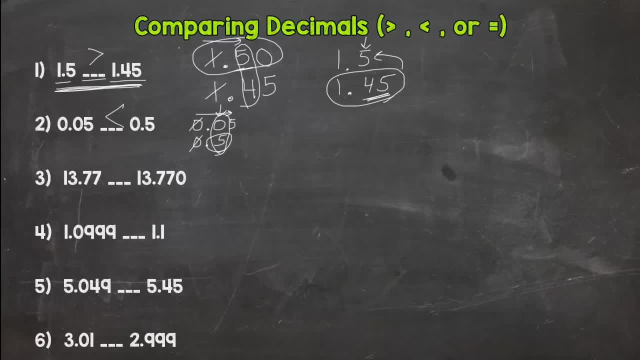 tenths is the greater number here, and you would read this: five hundredths is less than five tenths. All right, let's line up number three. I'll line it up over here. Thirteen and seventy seven hundredths can compare to thirteen and seven hundred seventy thousandths, So this is kind of. 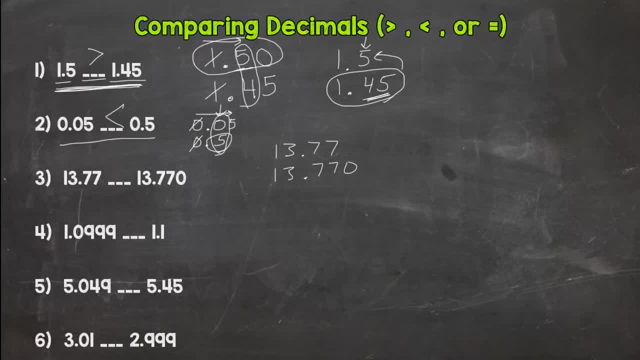 like number one. They don't line up directly, so we are going to put a placeholder zero on the top one here. so they both go to the thousandths And you probably recognize that they're the same thing. but let's go through our process here: left to right, Same in the tens, Same in the ones, Same in the tens. 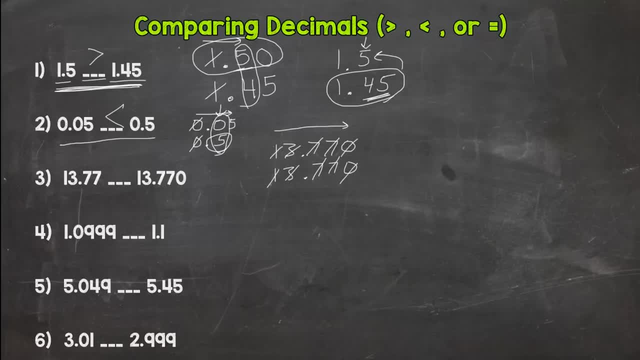 Same in the hundredths, Same in the thousandths. So these two decimals are equal or equivalent. I'm gonna rewrite them just for a common mistake here. It does not matter that this one has 770.. It has more digits or more numbers than the. 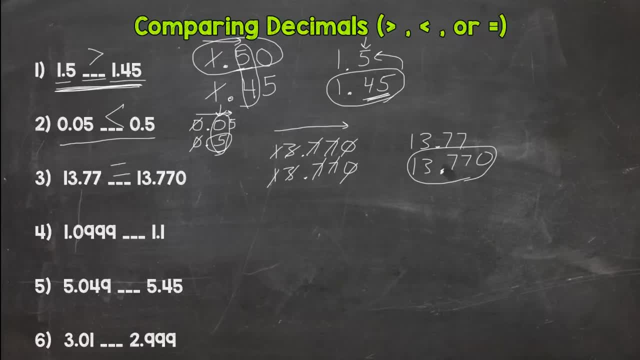 top one. When we talk decimals you need to go place by place and recognize that zeros to the right do not change the value of that number, So they are equivalent. That will come up again, so make sure you're. that's why I said you have to be familiar with equivalent decimals All. 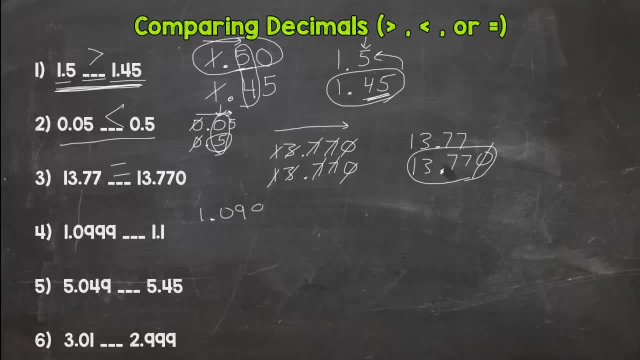 right number four. Let's line them up. We got a bunch of nines in this one and then we have one and one tenth. Now I put number four for a reason, because when students are starting out they say, oh, this one has a bunch of nines and 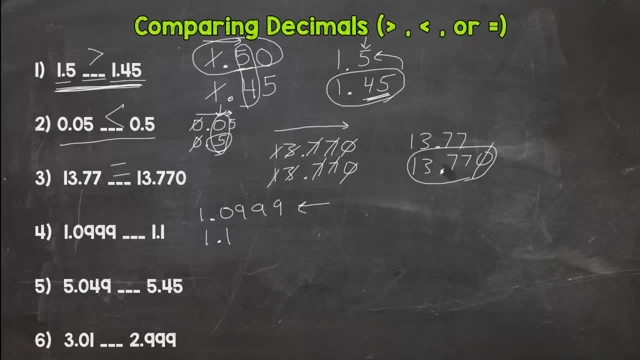 it has a lot more numbers so it's greater, Not true? You need to go through your process: Look left to right, going place by place. Can't compare wholes, so let's check tenths. Oh, we have a zero compared to a one here. This number is: 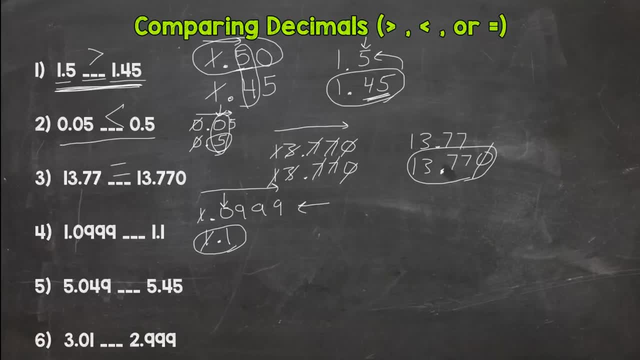 greater because of the tenths place. Go place by place. So you would read that one and nine are nine. wait, let me start over. One and 999. ten thousandths is less than one and one tenth. All right, let's do number five. Line them up. make sure we have these. 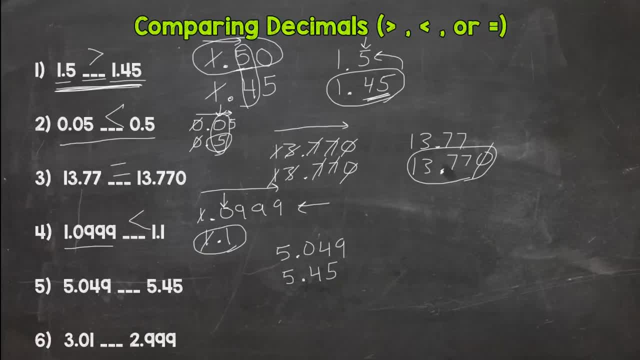 correct and you should be able to explain why. which one of these two numbers is greater. Can't compare the wholes, they're both fives. Ooh, it looks like we can pair. it can compare the tenths place and this four is greater. That makes the 45 hundredths greater than the 49 thousandths up there. It does. 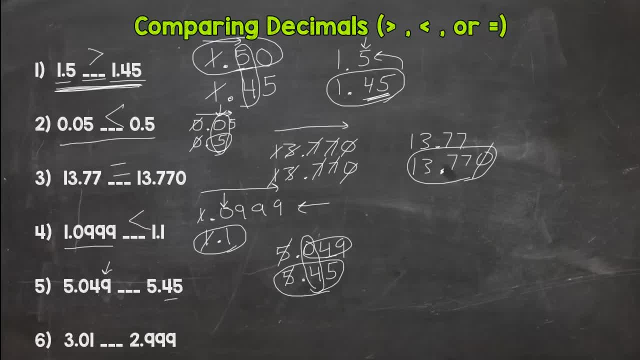 not matter that this is a 49. This 45 is greater value because of that four in the tenths place. So you would read this: one Five and 49 thousandths is less than five and 45 hundredths. And this is another one where we should have put a placeholder zero here. And then we 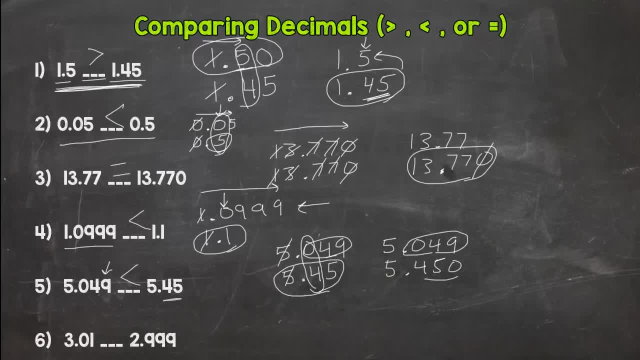 can see: oh, 49 thousandths, that's a lot less than 450 thousandths, right? So use those placeholder zeros. and then the last one I'm gonna write out. this is another common mistake. I see: Oh, this has a lot of nines. Look, let's look at. 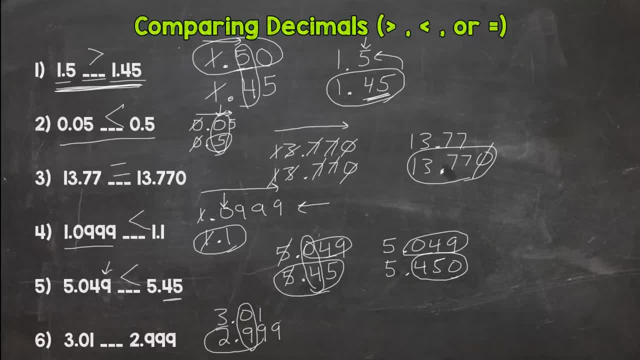 the tenths place, A nine is greater than a ten, So let's look at the tenths place. A nine is greater than a zero, so it must be this one automatically. does anyone see why it's not the nine, nine, nine, always check your whole numbers first, right, this has. 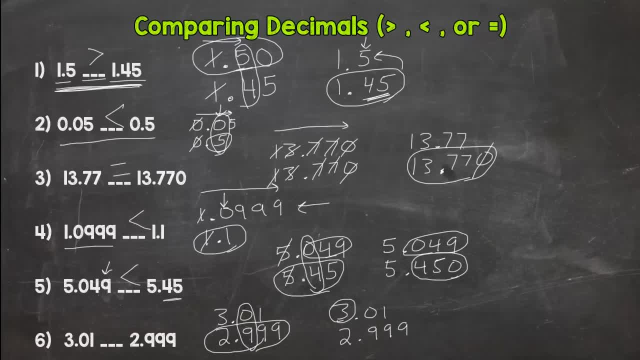 a three in the whole number, so it doesn't matter what this one has for a decimal right, three holes is automatically greater than two holes. go left to right, so three and one hundredth is greater than two and nine hundred ninety nine thousandths. so line your decimals up, go left to right use. 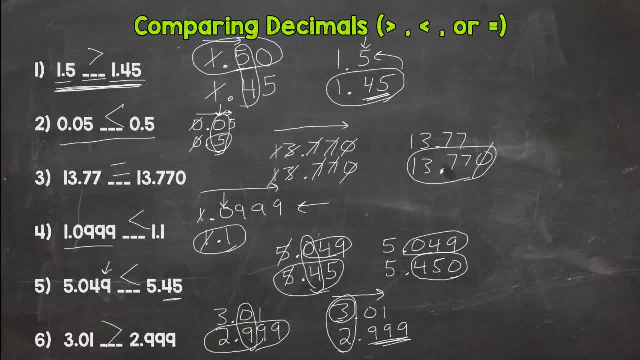 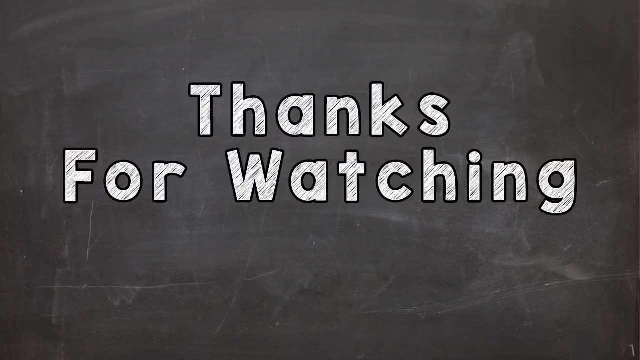 placeholder zeros if need be, and comparing decimals isn't too bad. so head over to the mastery check, and I have some over there that you are going to try on your own to see if you have it down. so see you at the mastery check. thanks for watching. please hit that subscribe button and drop a comment if 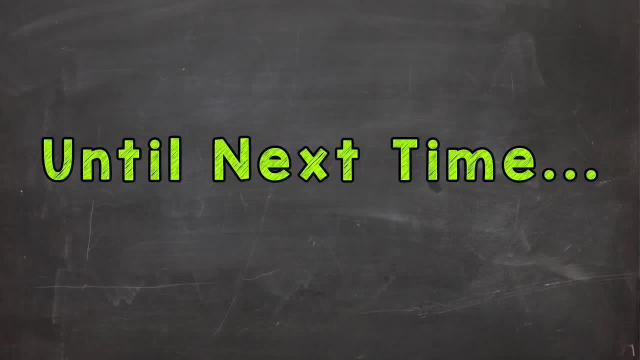 there's any material you'd like me to cover until next time, peace.